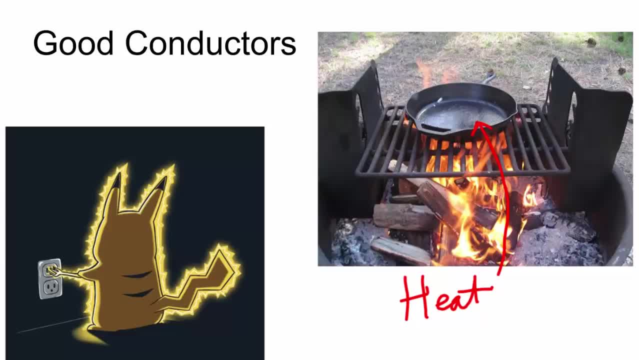 we can heat it up with this fire and it transfers that heat very well to whatever we might be cooking, Or they could be a good conductor of electricity, right. And so we can see here that Pikachu is sticking a metal fork into an outlet and he's going to get a good shock, even though 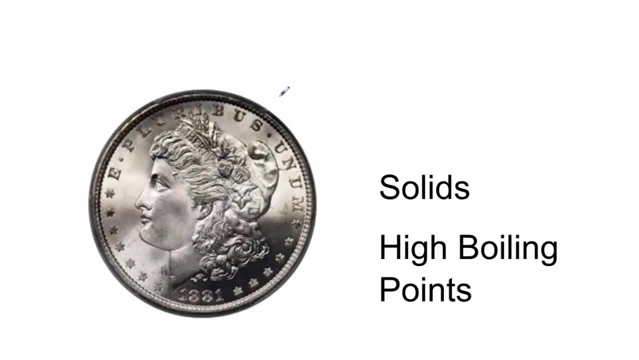 he is Pikachu. Metals are also shiny, right, And we might say luster as another way to describe shiny. They are almost all solids with the exception of mercury. at room temperature They have high boiling points, right, That's because they are those solids, all right. 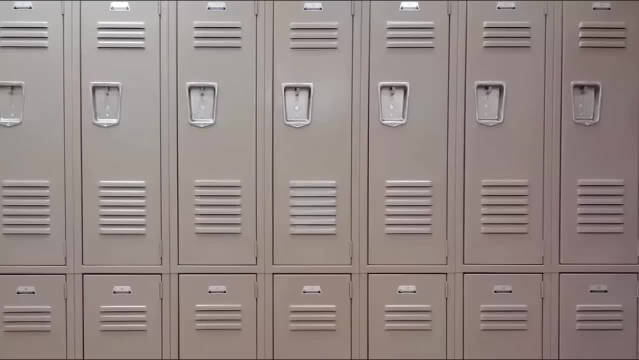 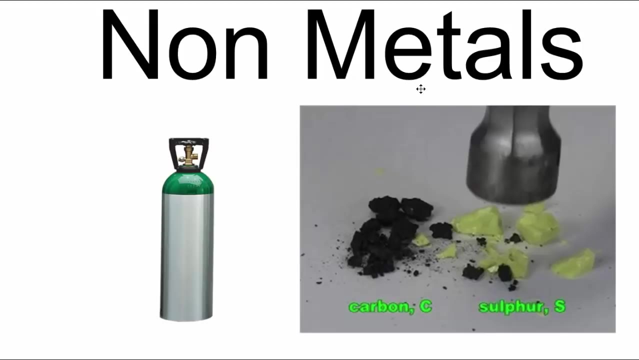 All right. metals like these lockers right here are also notoriously hard to break, So think about that. You wouldn't want to punch these lockers. It would hurt your hands because metals are hard to break. We already knew that. So nonmetals are the exact opposite. 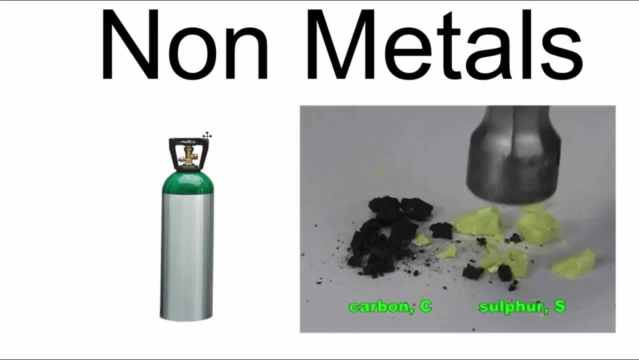 of metals. While most of the metals are solid, most of the nonmetals are gas And the ones that are solid, like sulfur and carbon. here they're very easy to break right, So we would say that those are brittle. So the solids are brittle, and most of them. 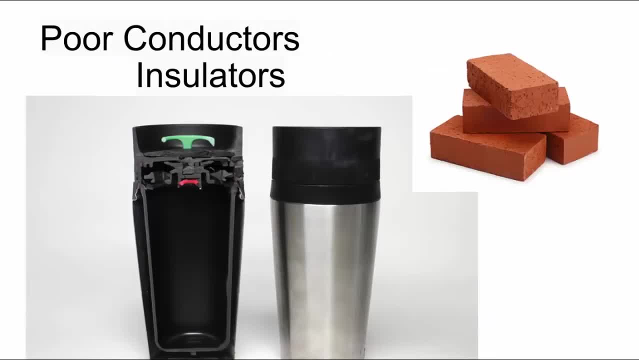 are gas. They are also poor conductors. okay, We would say that they are insulators. So we said most of them are gas. Look, if we use these kind of cups to help keep our coffee or hot drinks hot, notice what's in the middle of those cups. right there, right In this area, right in here. 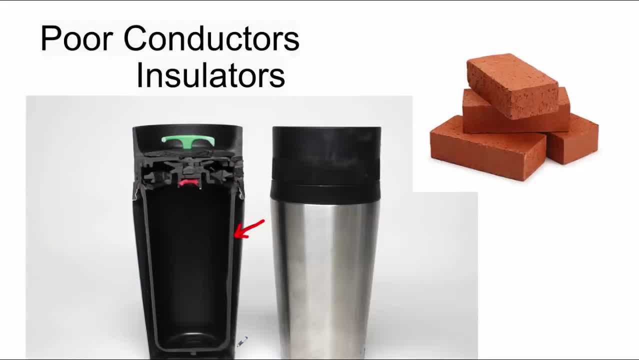 there's just a space, There's just air in there, right, And that air, which is made of gas, is a good insulator. It's a poor conductor of heat. It keeps the heat in here and doesn't let it pass through, unlike the frying pan, which passed that heat through pretty easily. okay, And they are. 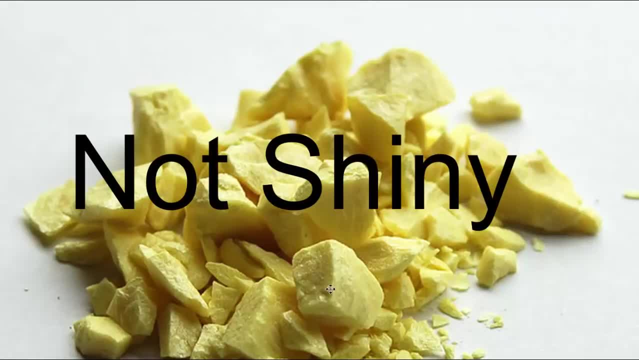 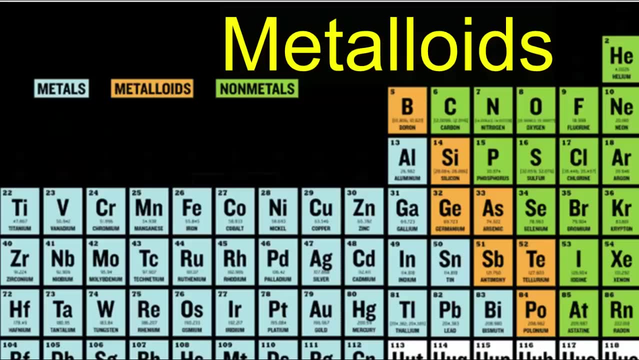 also not shiny. So here's some sulfur here. It's pretty dull, The ones that are solid carbon and sulfur. they're not very shiny at all. Metalloids are in between metals and nonmetals, both in characteristics and where they. 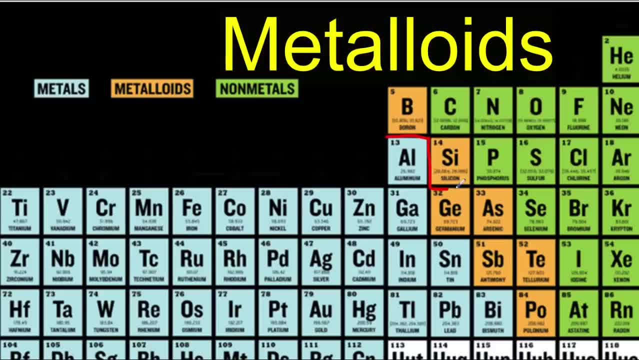 appear on the periodic table. So we say that there's that stair step, It comes right down through here And anything that's on that stair step is going to be a metalloid. The one exception is aluminum- right Aluminum- while it's on the stair step and it appears like it would be a. 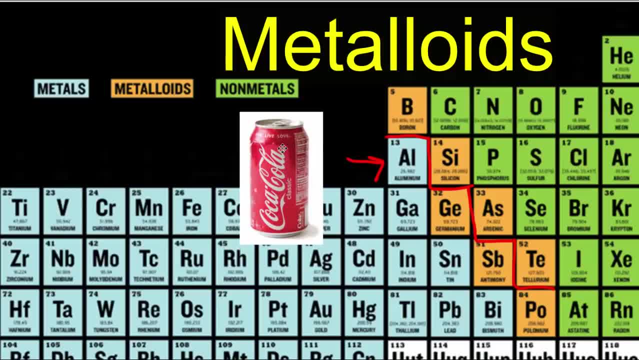 metalloid. think about it. We look at an aluminum can. Aluminum is a great conductor of electricity. It is malleable. It's been formed into thin sheets for these aluminum cans and it's definitely shiny. So it's giving you all the characteristics of a metal, But all the rest of them boron. 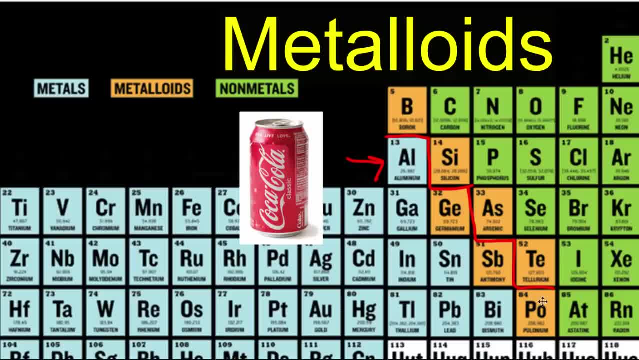 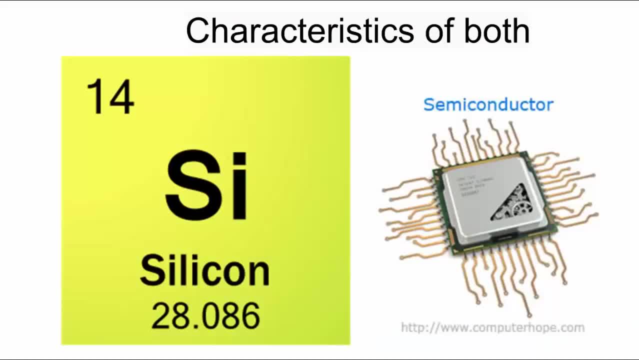 silicon, germanium, arsenic, antimony, tellurium, polonium- these are metalloids. Now metalloids are going to share the properties of both metals and nonmetals. Silicon is a perfect example of this, And the very fact that you're hearing my voice and watching this video right now is because 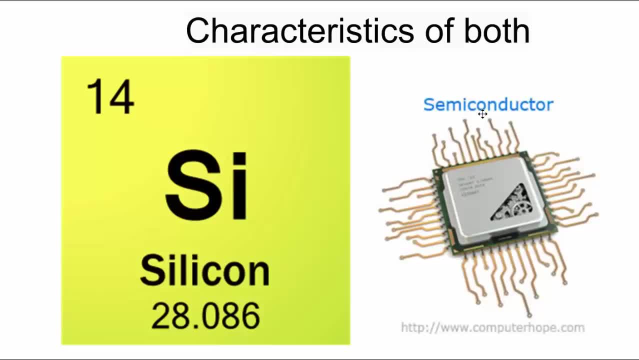 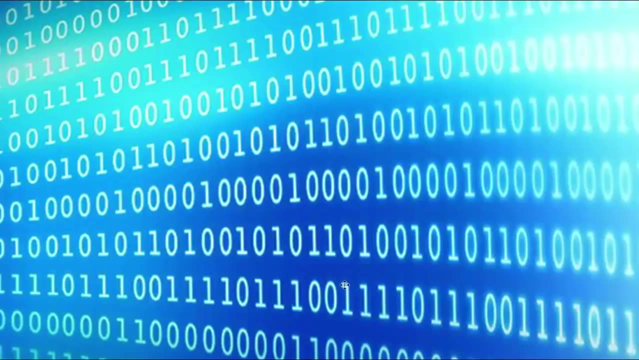 of silicon. Silicon is a semiconductor, which means that it is both a conductor of electricity and not a conductor of electricity. We can control that, And because we can control that, we can send information on off ones and zeros in a binary code. Well, this is how computers. 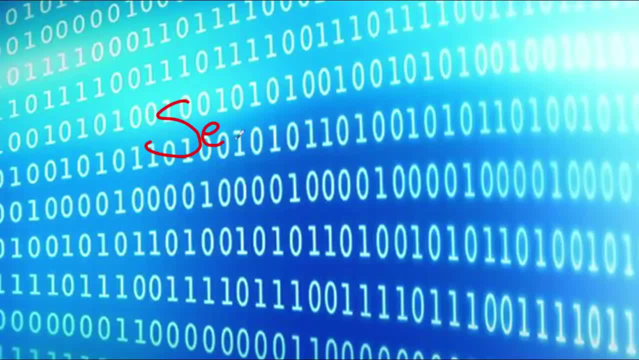 work in this binary code. So if we didn't have semiconductors that were in your phone or in your computer, then none of this would be possible. You wouldn't have an iPhone or a Galaxy It, just it wouldn't happen. So you are a huge fan of semiconductors and metalloids. 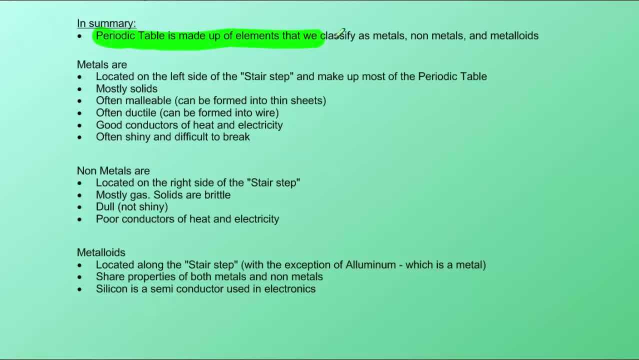 In summary, the periodic table is made up of elements that we classify as metals, nonmetals and metalloids. The metals are located on the left of the stair step and they make up most of the periodic table. Metals are mostly solid. They're often malleable. 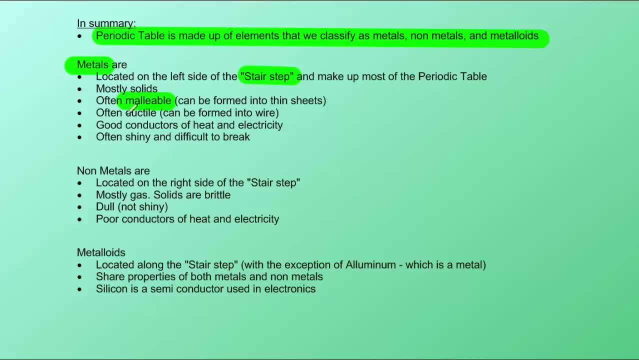 which means they can be formed into thin sheets. They're often ductile, which means that they can be formed into wire. They are good conductors of heat and electricity. And they are good conductors of heat and electricity. They're often shiny and difficult to break. 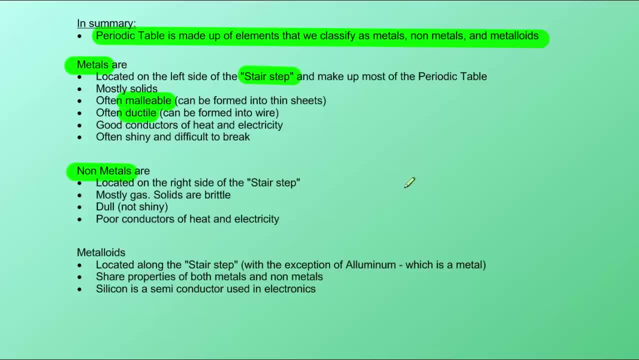 Nonmetals are located on the right side of the stair step. Most of them are gases. The ones that are solid are brittle. They're dull, not shiny, the exact opposite of the metals. They are poor conductors of heat and electricity. We call that property. they are insulators.